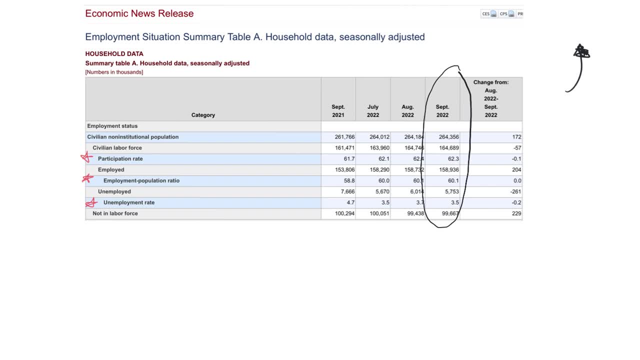 the most recent data, which is September of 2022, to calculate the three items that we are interested in. Let's start with the unemployment rate. We know the unemployment rate equation is the total number of unemployed over the labor force. Multiply that by 100 to get it into a rate. 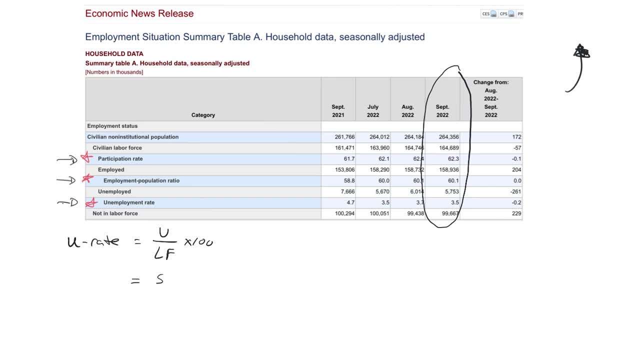 Let's go ahead and take the data that we have here. Our unemployed is 5,753, and our civilian labor force is 164,689.. Multiply that by 100.. I go ahead, I plug that into my calculator and what do I get? 3.49%. And what do we see up here? 3.5, because it was rounded. Check We. 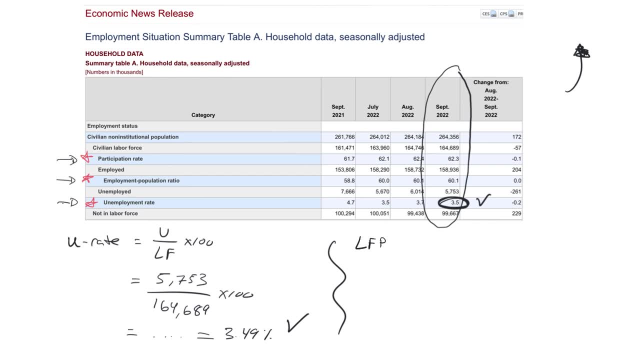 got it. Now let's do the labor force participation rate, which we know is my labor force divided by my working age population. My working age population here is going to be denoted as the civilian, non-institutional population. We won't get into exactly what that means here, but just 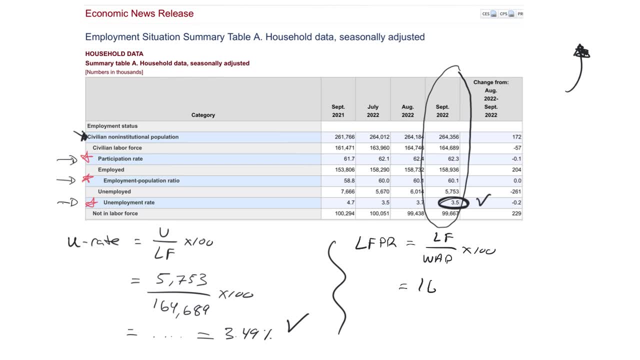 know that we're going to be looking at my labor force, which is 164,689, and divide that by that population, which is 264,356.. Multiply it by 100 to get it into a percentage I'm going to plug. 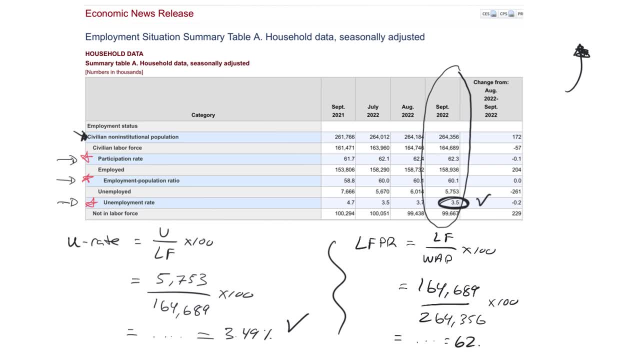 that into my calculator and what do I get? 62.29%, And I look up here: 62.3.. Again, we got that right. I'm going to move this slightly, make it a little bit more, and I'm going to go ahead and take the. 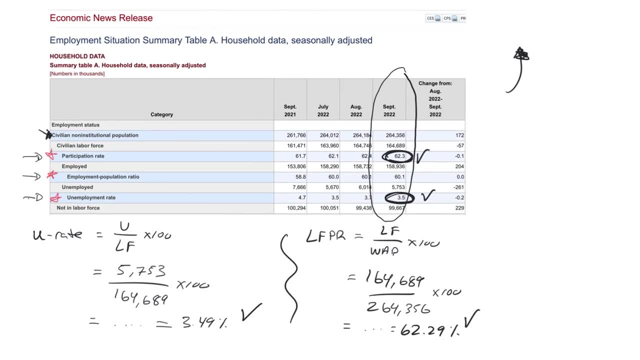 little smaller so we can do the employment to population ratio. So over here we know my employment to population ratio is just going to equal that total number of employed over that population, Again multiplied by 100 to get it into that rate that we're looking for Employment. 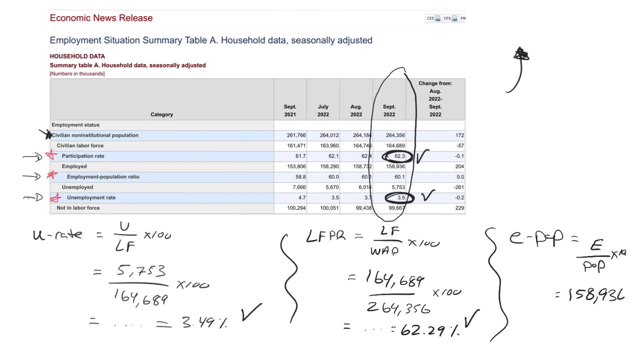 up here we see, is 1, 5,, 8,, 9,, 3, 6, divided by that population: 2, 6,, 4,, 3,, 5,, 6.. And what do we get when we plug that into our calculator? 60.12%, Oh, 60.1.. Yep, we got that.